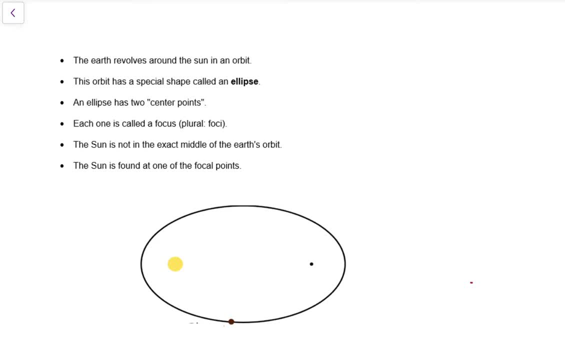 The ellipse, the oval itself and the two foci or the two focus points in the center of the ellipse, And then we will label the two foci. Another important part of the ellipse that we need to learn to identify is what's called the. 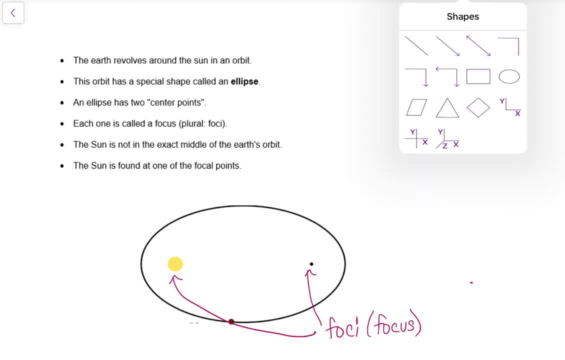 major axis. So in this case the major axis is the line that goes directly through the center of the ellipse, straight through the two foci points. So the major axis starts at the edge of the ellipse, it runs straight through the two foci points. 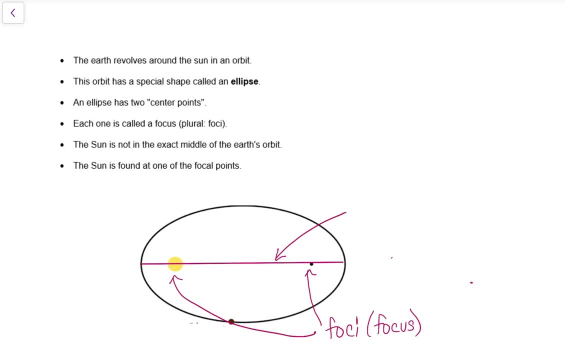 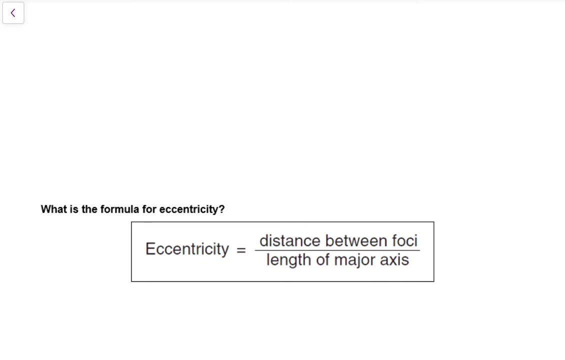 And ahead to the and goes straight through to the other side of the ellipse. Those are the major, important parts of the ellipse that we need to know in order to calculate the eccentricity. So before we can learn to calculate the eccentricity, we need to learn the formula. 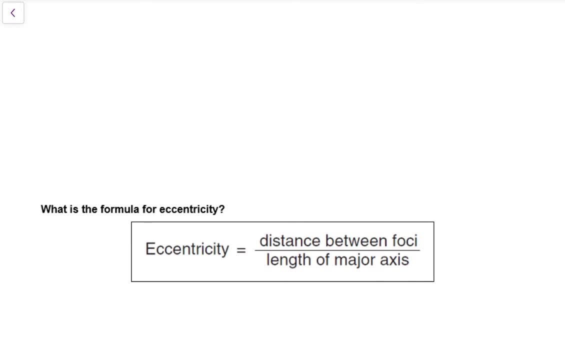 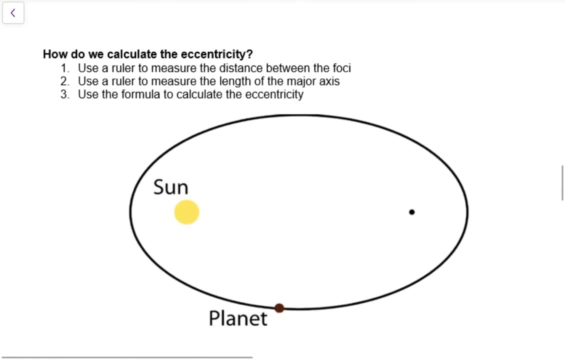 The eccentricity is equal to the distance between the foci divided by the length. How do we calculate the eccentricity? First, we will use a ruler to measure the distance between the foci. So remember, the foci points are those two eyeballs, those two dots in the middle. 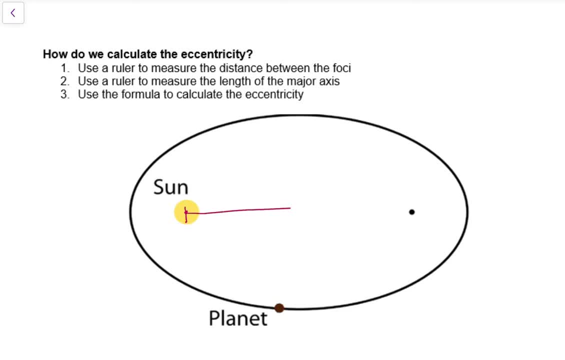 So the distance between the foci would be the distance between them And in this case you want to aim to measure exactly in the center of the dot, Step 2.. We will use a ruler to measure the length of the major axis. The major axis is going to be the line that goes from the edge of the ellipse straight. 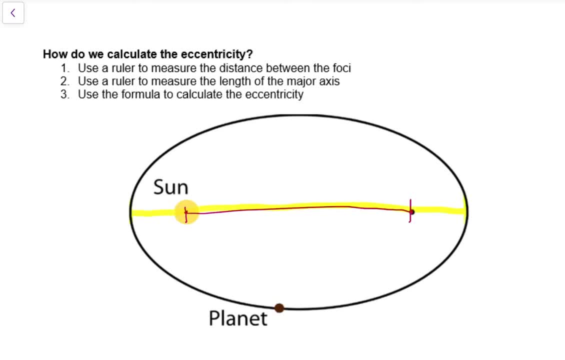 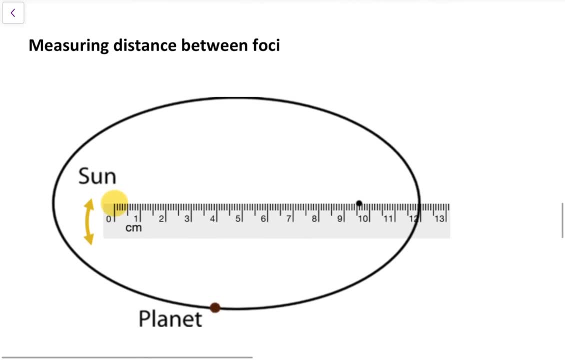 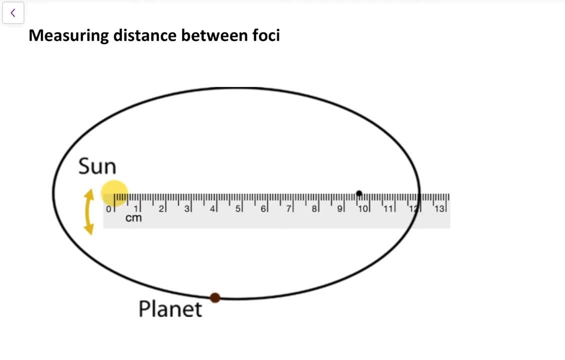 through the foci across all the way through to the other edge of the ellipse, And then we would use the formula to calculate the eccentricity. Let's do this step by step. In this case, if we want to measure the distance between the foci, 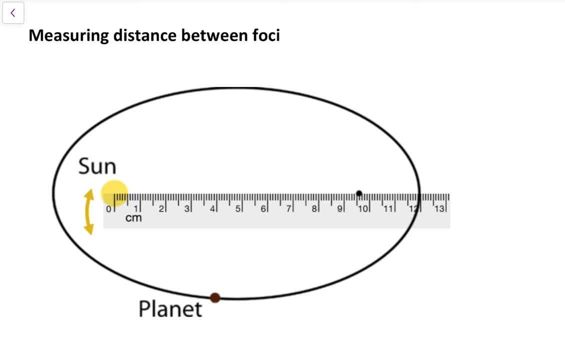 We are going to line up the zero line of the ruler. Ok, so the first line of the ruler, Not the edge of the ruler over here. but you are looking for that zero mark, The zero, the very first solid black line on the ruler. 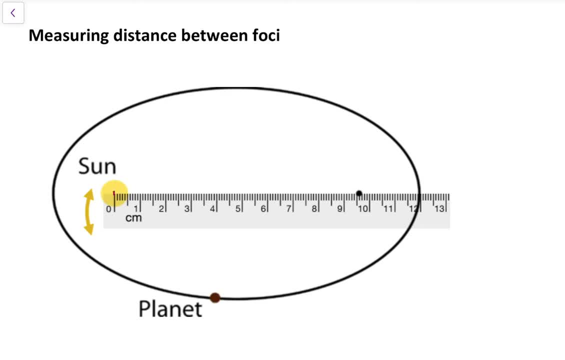 And you want to line that up as close as you can to the middle of the first focus point, And then we are going to measure all the way across until the center of the second focus point, Right about here. So in this case I am measuring to the nearest tenth of a centimeter. 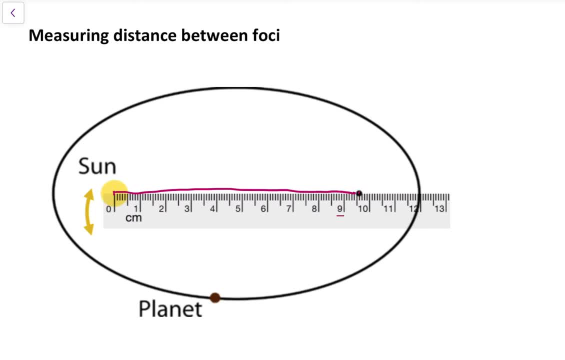 Here is 9 centimeters. Each smaller line represents 1 tenth, So this would be 9.1, 9.2, 9.3, 9.4, 9.5.. And it looks like it measures up to be about 9.6 centimeters. 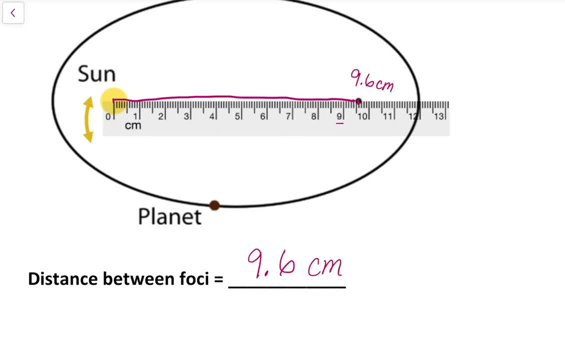 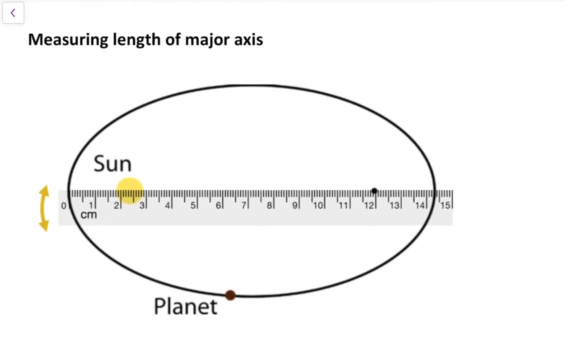 Distance between the foci equals 9.6 centimeters. Next, I need to measure the length of the major axis. Now I am going to take my ruler and take that first solid black line representing the zero mark, and move it to the very edge of the oval. 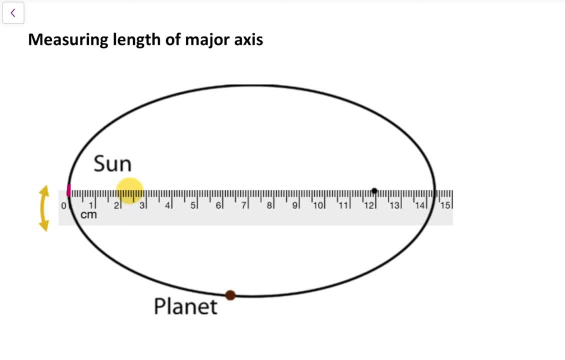 The farthest edge of the oval. You want to make sure your ruler is running straight through the center of the foci. That way you know that your ruler is in the middle of the ellipse. We are going to measure all the way across. 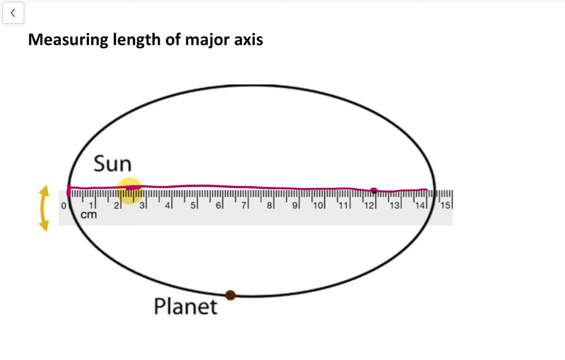 We are going to measure all the way across, Straight through, to the opposite edge of the ellipse, Straight through to the other edge of the oval, Again to the nearest tenth. In this case, here is 14,, 14.1,, 14.2.. 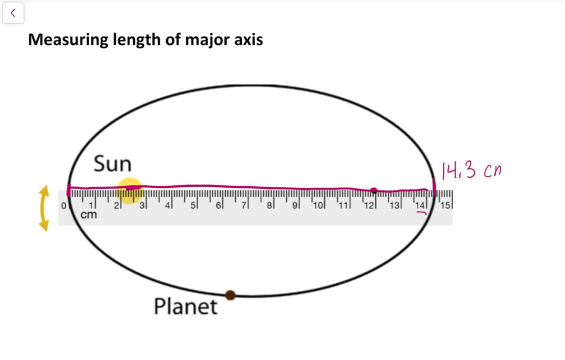 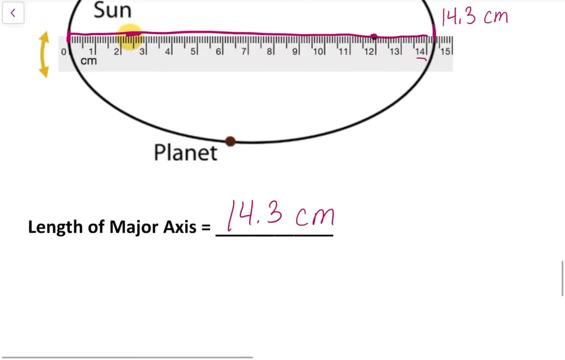 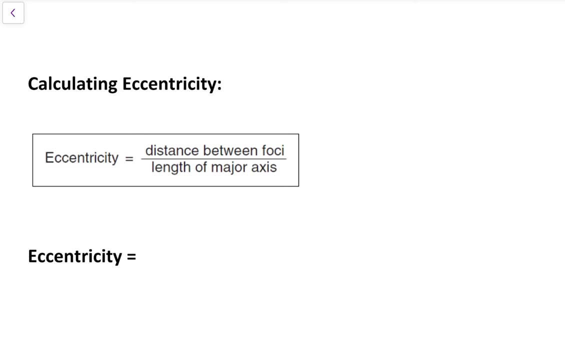 It looks like it is about 14.3 centimeters. Length of major axis equals 14.3 centimeters. So if we want to calculate my eccentricity, the formula for eccentricity is equal to the distance between the foci divided by the length of the major axis.